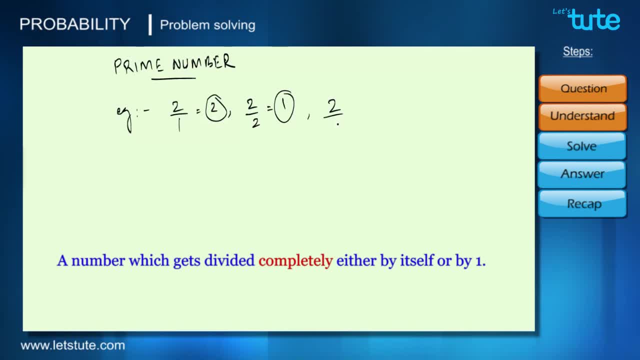 be completely divided. But if we divide 2 by any other number, let's say 6,, then we get 1 upon 3.. Or by 3, then we get 0.6.. Which is not a complete division. So 2 can only. 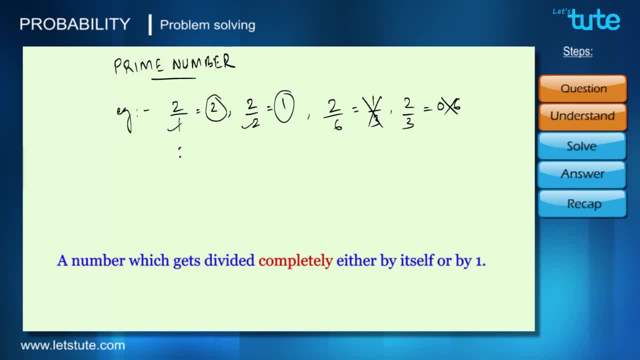 be completely divided, either by itself or by 1.. Similarly, 3 can be divided by 1. It can be divided by itself, But if we further divide it with any other number we get fraction or it cannot be completely divided. So 3 is also a prime number. Like that. we have a list of prime numbers which can be. 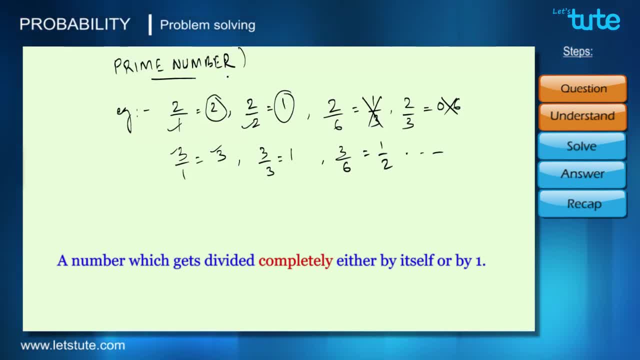 divided by itself or by 1.. So we have to not only find a card with prime number, but it should be less than 10.. So the prime numbers less than 10 will be 2,, 3,, 5, 7.. The next: 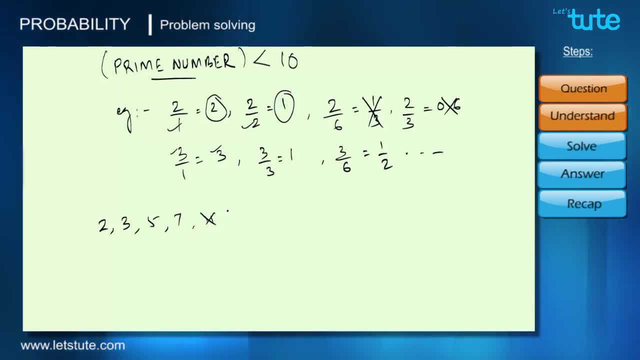 prime number is 11, which we cannot take as it is more than 10.. But, if we remember, we have cards starting from number 5, which means we cannot really take 2 and 3 as well. So there are 2 prime numbers that we require for this particular. 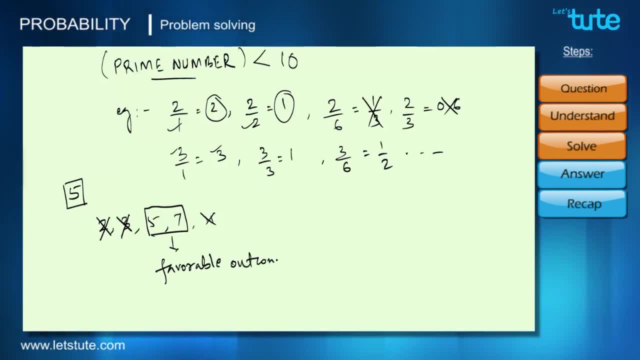 event. So these are going to be the favourable outcomes. And how many number of cards do we have, Since it starts from 5 to 50, that means cards 1,, 2, 3 and 4 are not there, Correct. So total cards that we have are 50 minus 4, which is 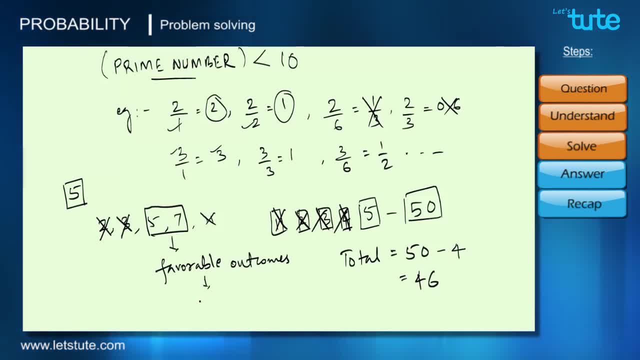 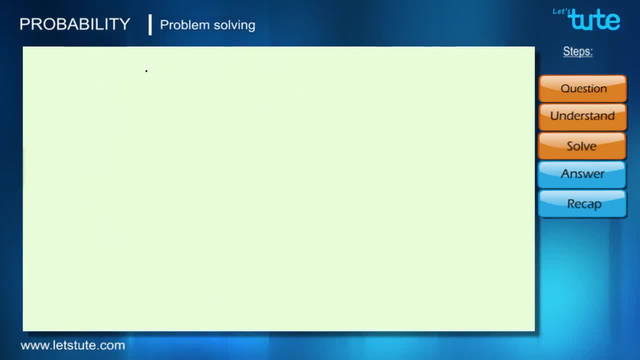 equal to 46. So we have 2 favourable outcomes and we have 46 total possible outcomes. Now we will substitute the same in the probability formula, And we have already studied the probability formula, for any event can be given by the ratio of number of favourable outcomes to 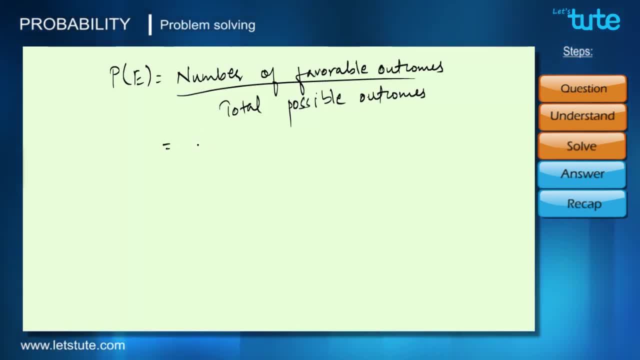 the total possible outcomes. So number of favourable outcomes were 2 and possible outcomes were 46. So the probability of drawing a card which is a prime number and less than 10 is 1 by 23.. Secondly, we had to find the card which had a number which was a perfect square Before.